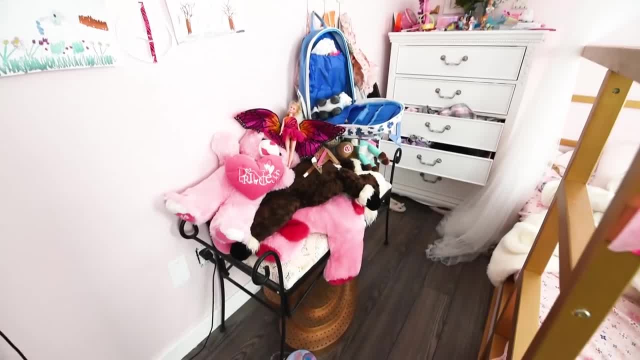 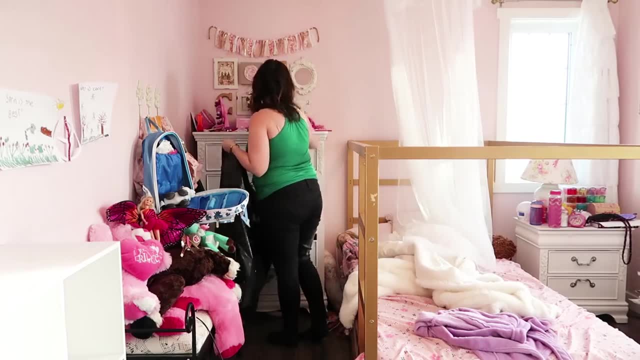 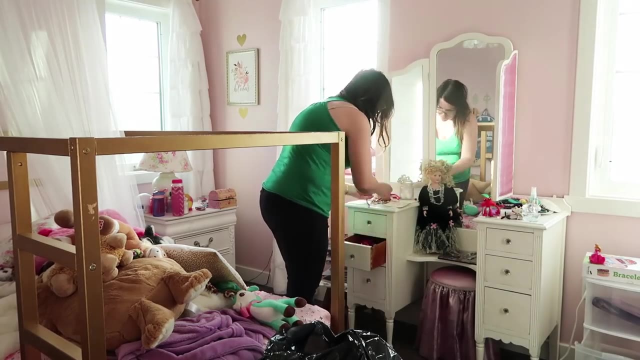 And then we have this old bench with a whole bunch of stuffed animals piled up. So first things first, I just went in there with a garbage bag and just tossed everything that she hadn't played with, that wasn't recyclable or donatable, And then I just went through and organized everything. 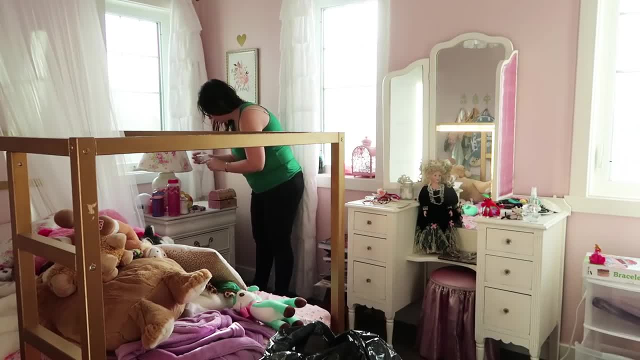 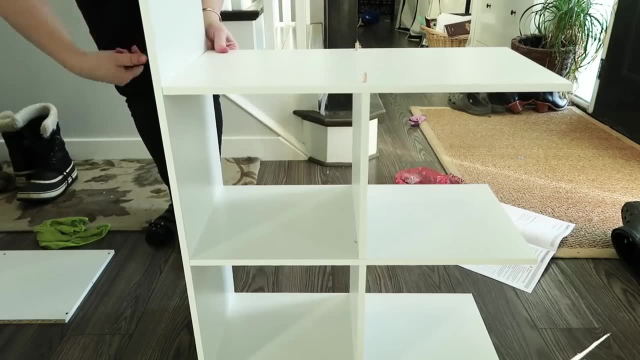 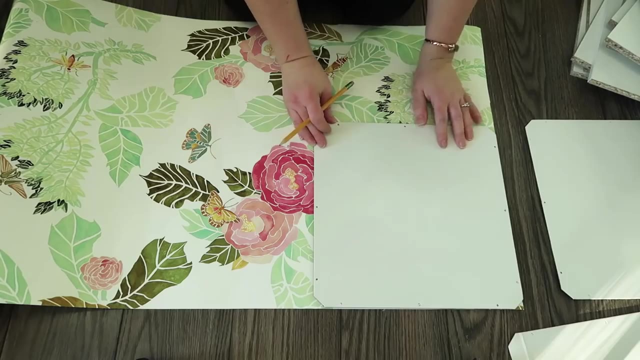 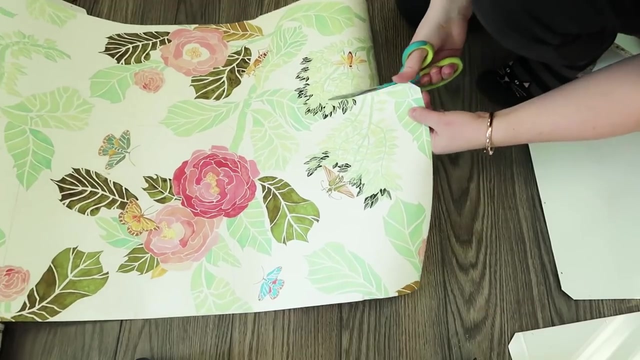 So put things in their places and purged and cleaned And then I just got an inexpensive cube shelf from the hardware store and put that together And then to personalize it for little C, I had this leftover wallpaper And I just cut it out to match the back squares of the shelves. 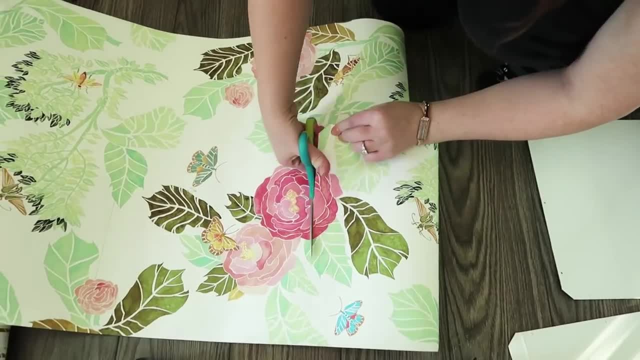 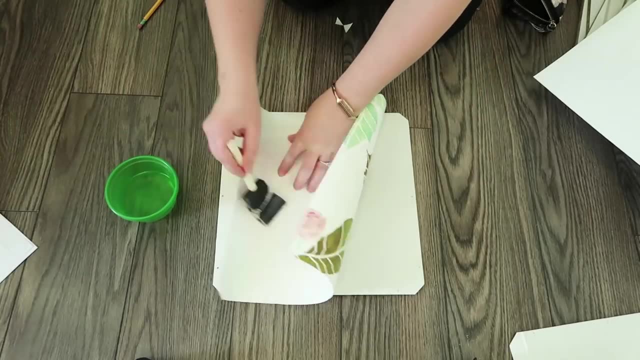 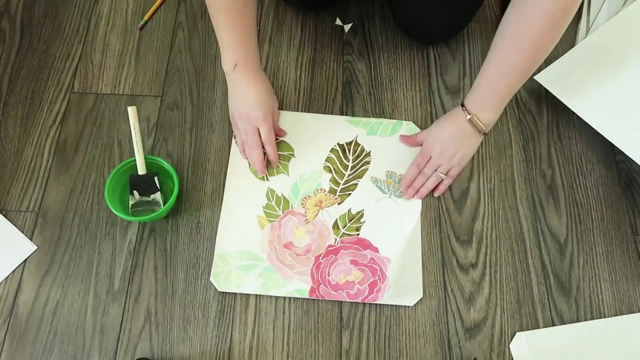 And then, after I cut the wallpaper out to match the backing of the shelves, I just took a foam brush and I just brushed the back with some water. This is pre-pasted wallpaper, so I just activated the paste with my foam brush And then just smoothed it onto the backing of this cube shelf. 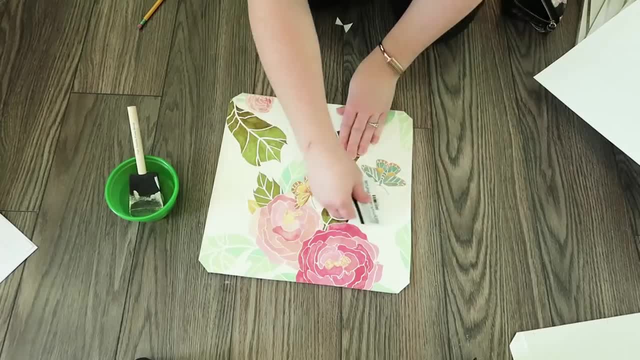 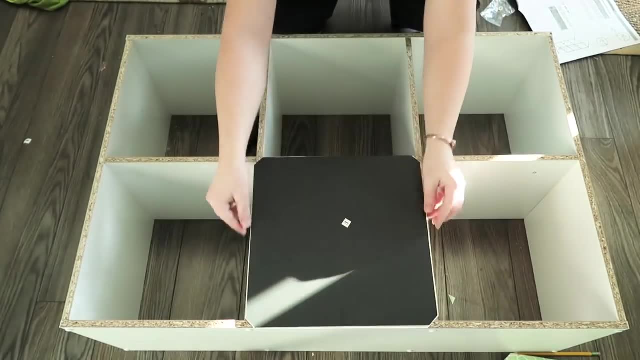 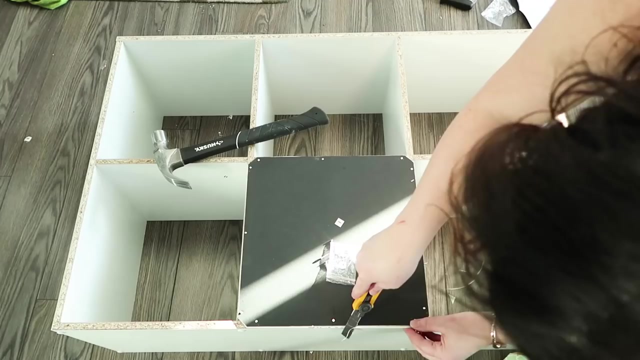 And I just used a credit card. And I just used a credit card to smooth out wallpaper after that. Then I nailed this backing onto the back of the shelf And there were three of these square backs, so I nailed three of them onto the cube shelf. 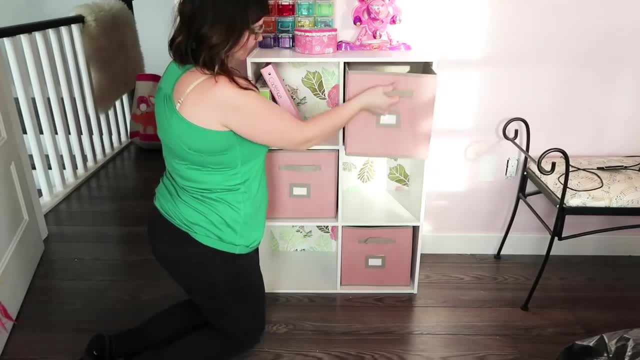 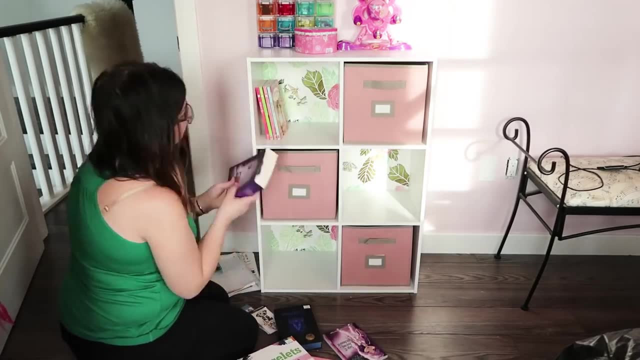 And then I just took a knife to take off any excess wallpaper. So I just got these fabric bins and they have some small crafts and some Barbies and her maple-y doll items, And then I was able to organize all of her novels in the rest of the shelf. 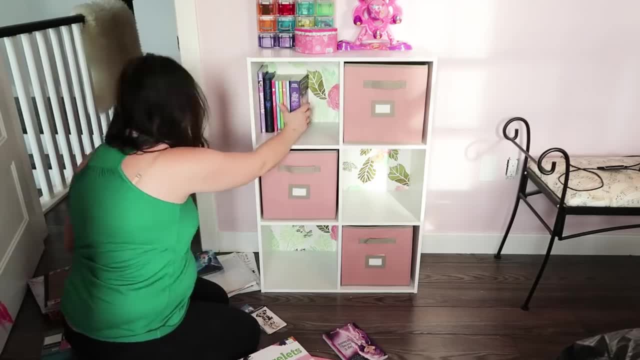 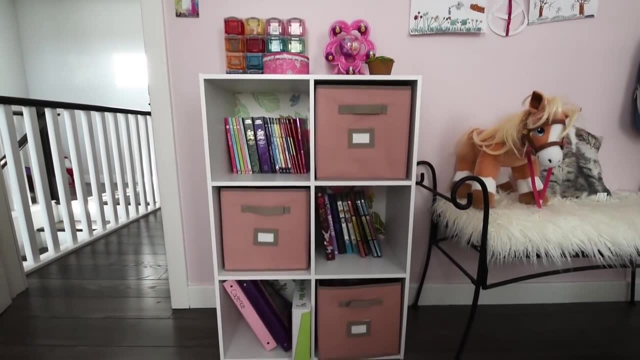 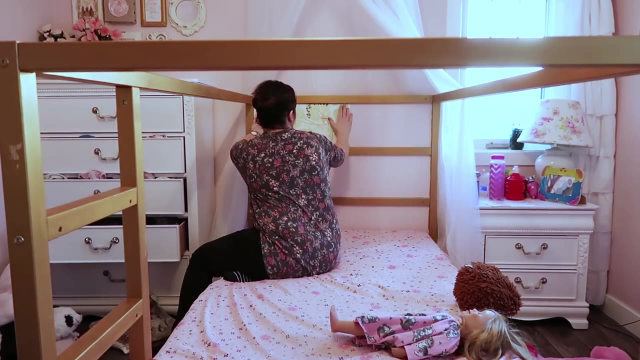 So I like organizing books by height, So tallest to shortest books. It just makes everything look just really nice and visually appealing. And now she has a cute little space for all her books and small toys. I wanted to carry this new wallpaper theme throughout the room. 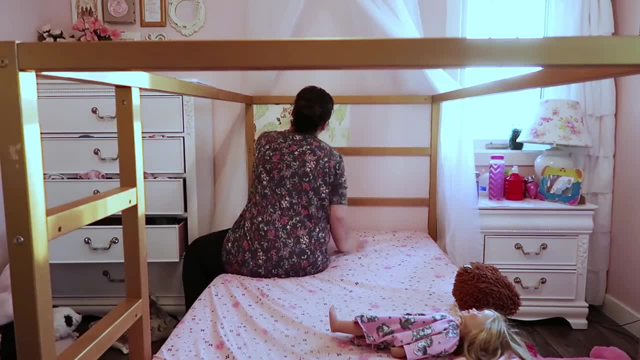 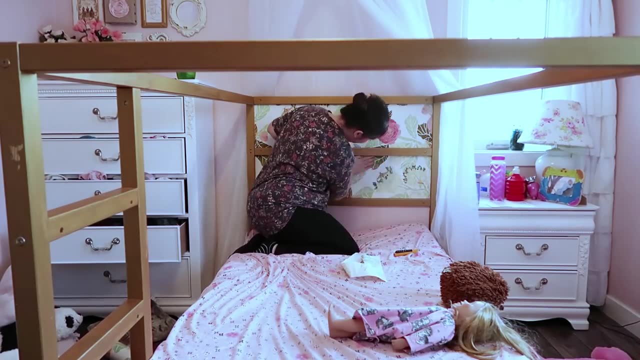 So another thing I did with the scraps of wallpaper is I put it on the back of her bed. I had painted this bed a couple years ago And I thought it was just a great way to kind of even give it more pizazz. 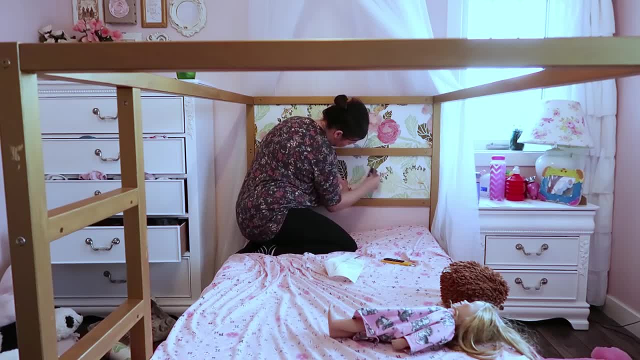 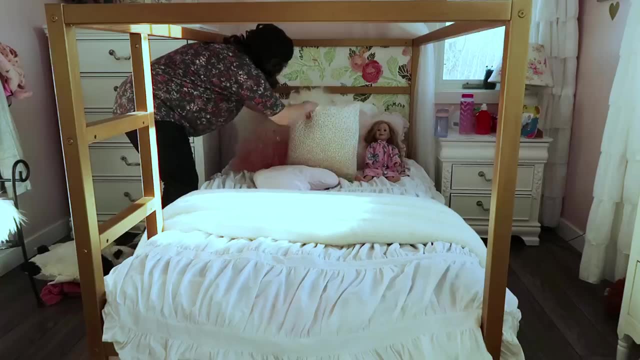 I get so many questions about this bed. It is a bunk bed that we flipped upside down. That's why it has the ladder on the side. And, yes, it is getting a little small for little C, So eventually we'll replace it. 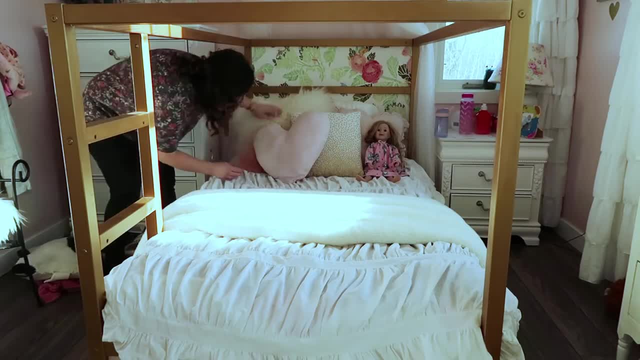 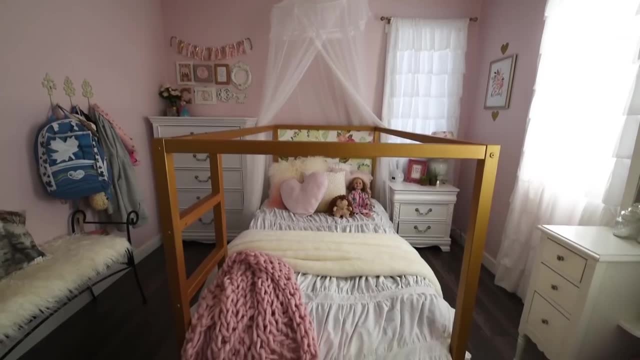 But I thought this was a really cute way just to kind of give it a little bit of an update for her. Most of the cushions on the bed I made myself And I'll leave a link in the description box below if you want to make the cushions and the bedspread as well. 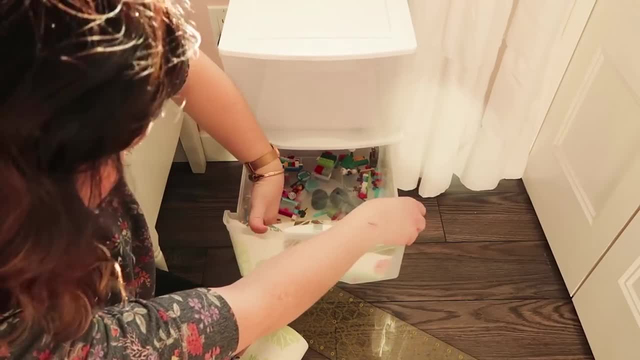 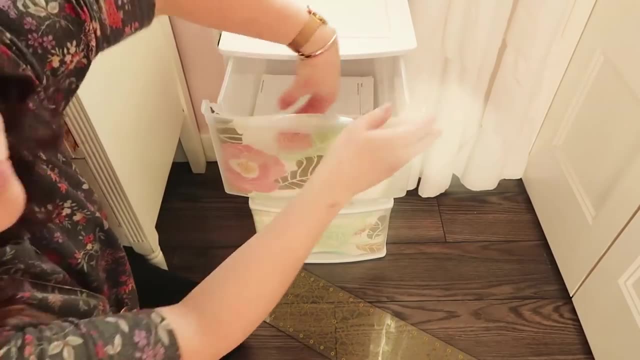 Then I just made the bed- I just had one of these just really small plastic organizers And popped some scraps of wallpaper into the drawers Just to give it a little bit of extra style And just again to bring this wallpaper theme to another spot of the room. 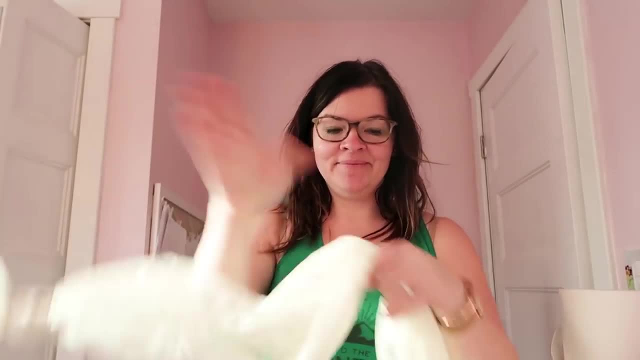 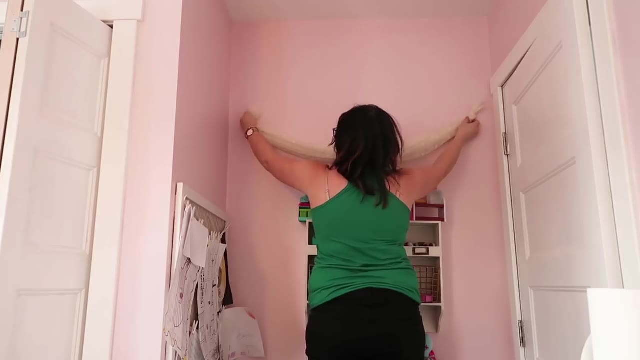 And this has all her Lego inside. I also took a scrap of lacy fabric And I tied two knots in each end And I took some command strip hooks And I put the hooks through the knots of the fabric And I hung it on the wall in this little corner. 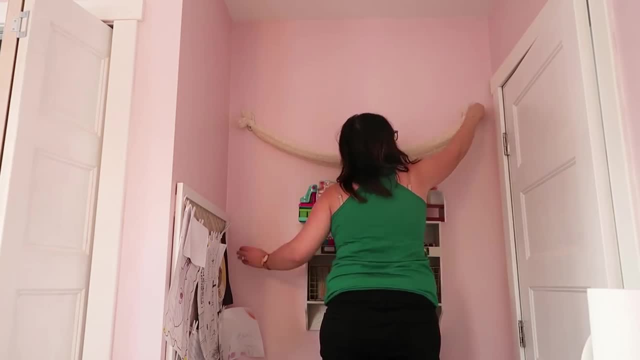 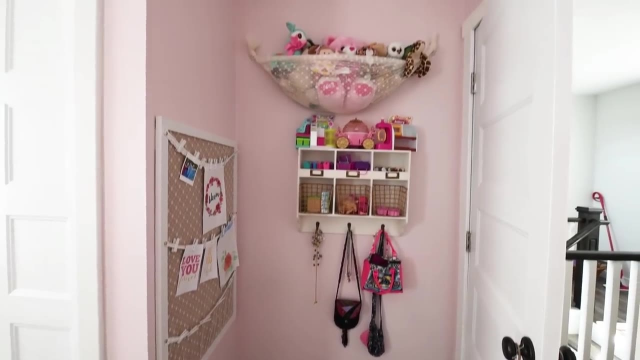 And this is going to act as a little stuffed animal hammock for little C stuffed animals. I've also seen these done in a triangle shape in the corner as well, But I just had enough fabric to do this way And it looks super cute. 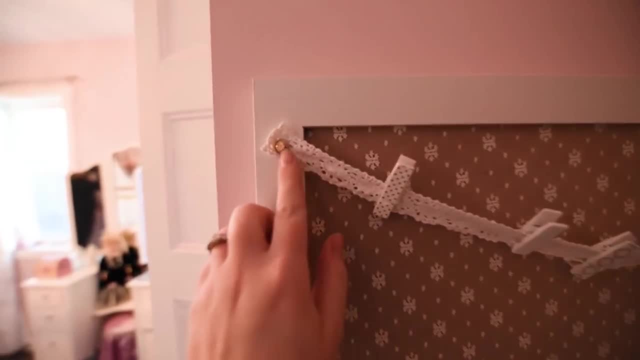 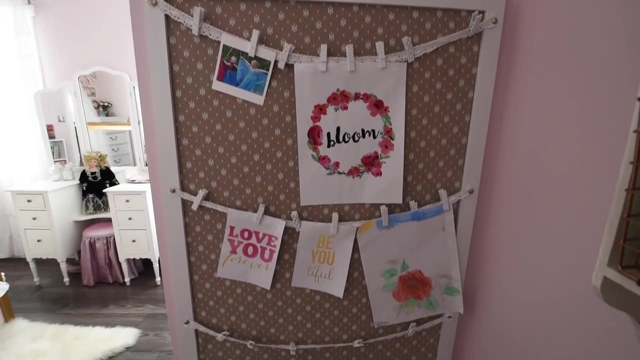 You might remember this little board I did before And it's just a picture frame And I put some lace inside And tacked up some lace trim and some clothes pins And it's a great place for little C to hang up her art. 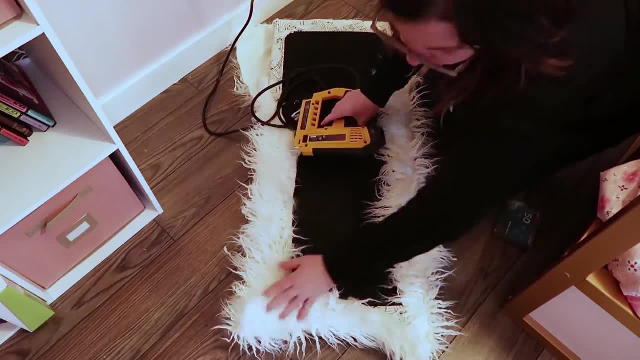 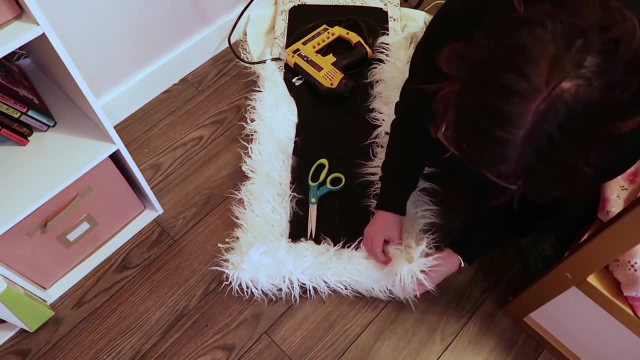 One final project I did in here was recover the old stool that she had in here, The old bench. I just had some leftover faux fur fabric And wrapped it around the cushion of the stool And used an electric staple gun just to tack that on. 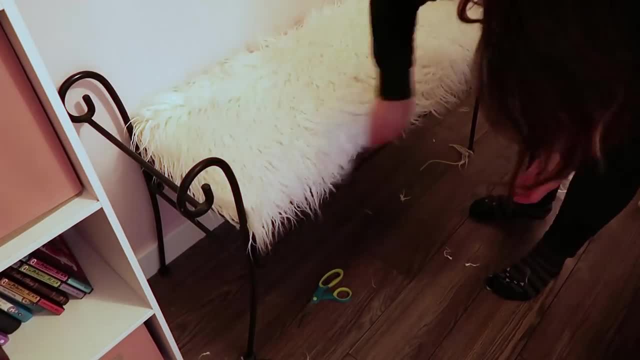 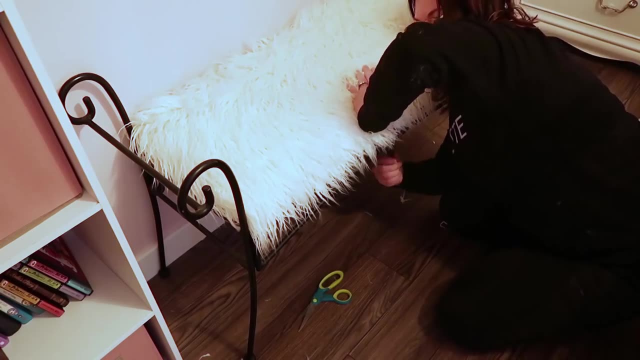 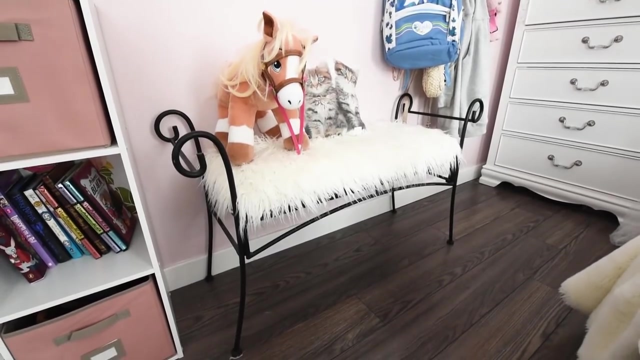 And then I popped it back on the bench just for kind of a nice little improvement, And it looks so cute and cozy. in little C's room She picked out this faux fur fabric And it's so cute, And it's so cute. 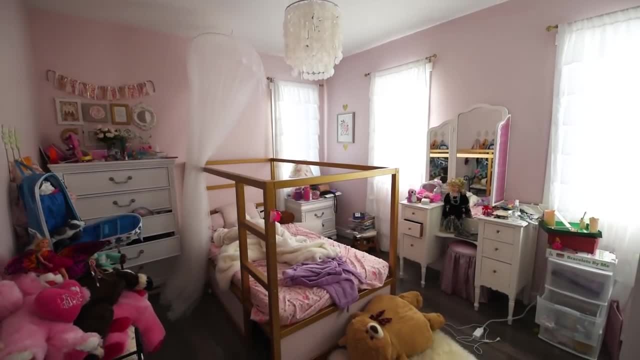 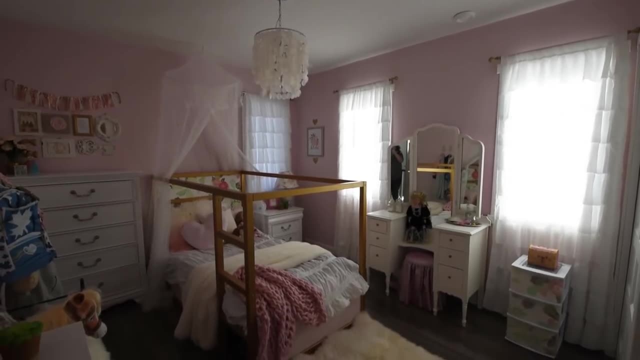 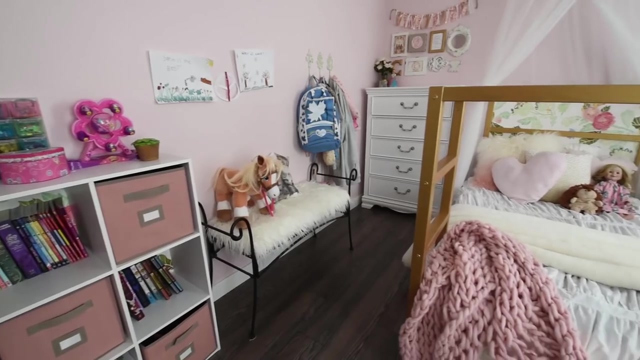 So again, here is how little C's room looked before we cleaned and organized it, And here's how it looks now, And I think it looks so much better. She is incredibly happy. I'll leave a little clip of her having a look at the first bit of the organization at the end of this video.